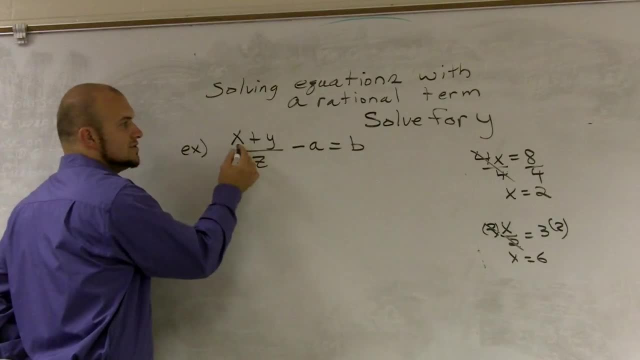 However, what you have to notice is there's two terms on the side. There's an x plus y over z and there's an a. So if you're going to multiply by z right now, you have to multiply by the z, by the x plus y and the z by the negative a. 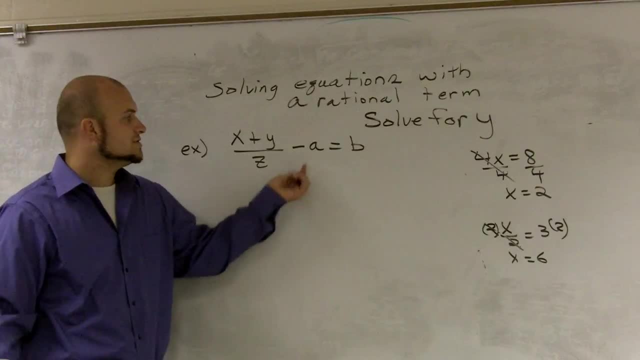 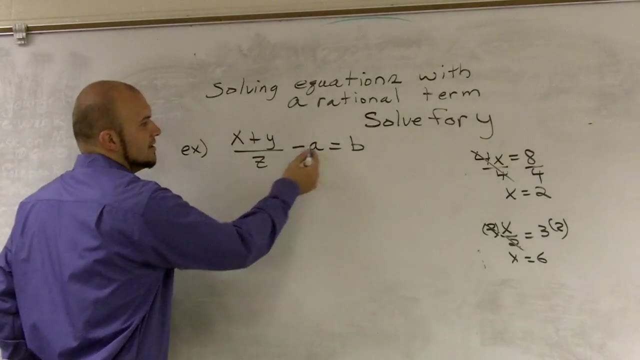 All right, I'm going to put the a onto the other side and then multiply by the z. It doesn't really matter which way you go, but to me this seems like the easier process. So I'm going to add an, a, because that's the inverse process of. I'm sorry, that's the inverse operation. that a is subtracted from our variable we're trying to solve for. 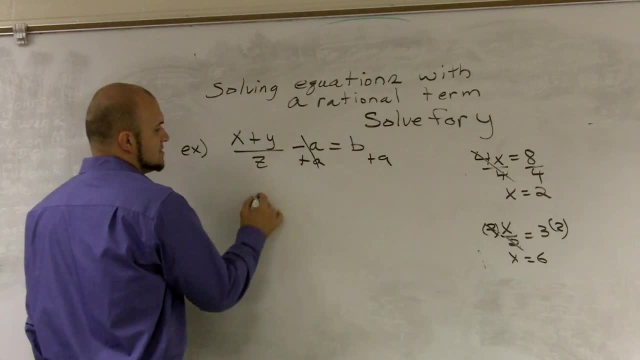 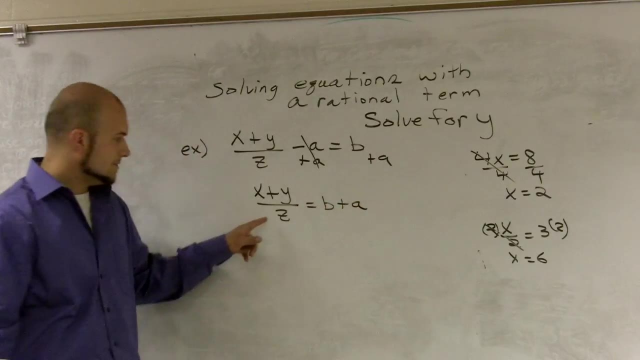 So I'm going to add the a. That's going to cancel out and become 0. So therefore, I'm going to have x plus y over z equals b plus a. Now I'm going to go ahead and multiply by my z. 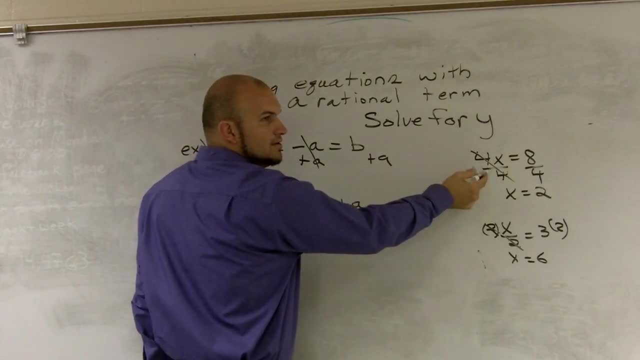 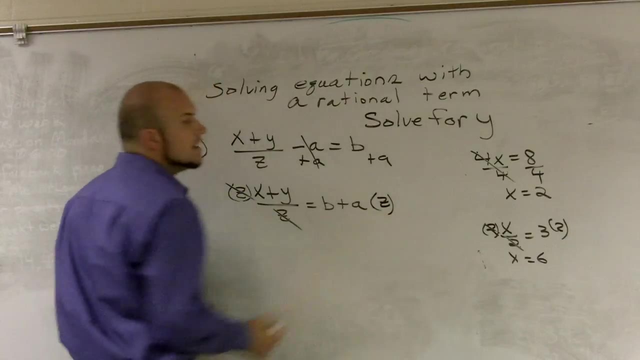 And what I notice is, just like over here, 4 over 4 equals 1.. z over z is going to equal 1.. So they really did cancel out. Then I multiply by z. on this side, Again, we have to be careful though. 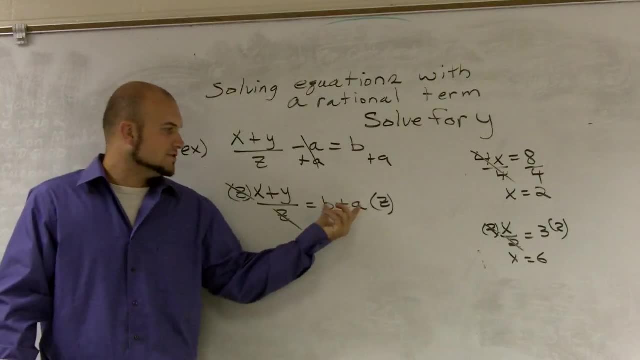 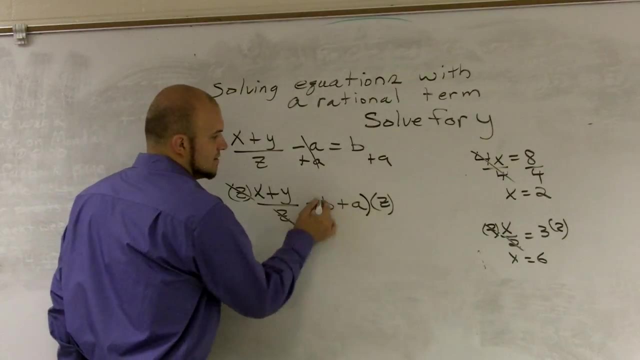 When we multiply, when we show that we're multiplying z on the side, we have to notice that there's two different terms. So you're not multiplying the z just by the a or the z just by the b, But we have to put parentheses around that b. 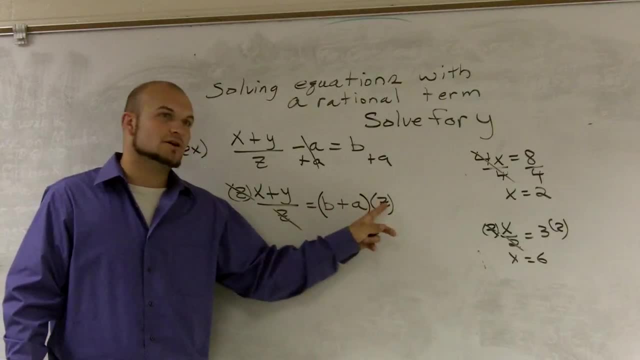 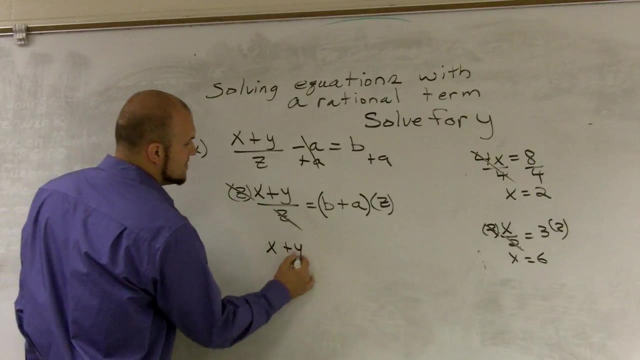 So we're going to do z over a to show that we're multiplying that z times the b and multiplying that z times the a. So therefore that cancels out. Now we're left with x plus y, And we usually like to represent this with a single term in front of the other two terms. 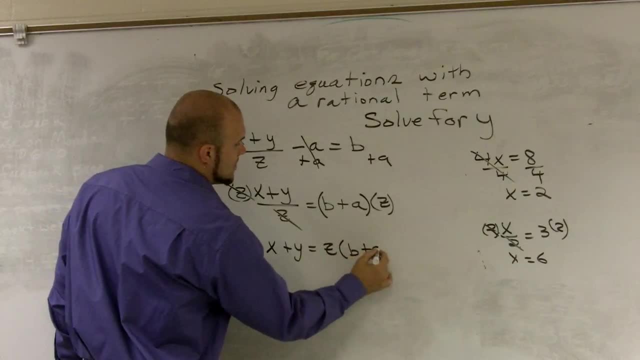 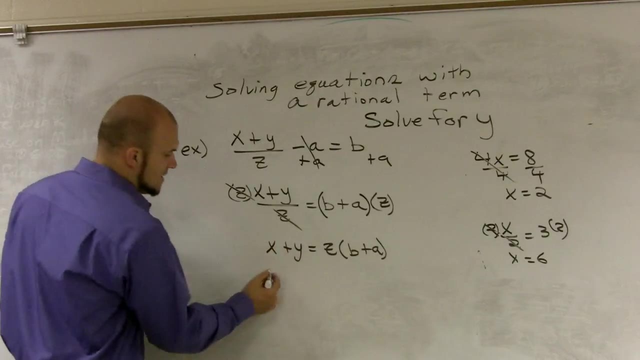 So I'm going to write z over b plus a, Then now, lastly, I need to get that y by itself, So I need to get rid of the x. Since the x is added to the y, I'm going to subtract the x. 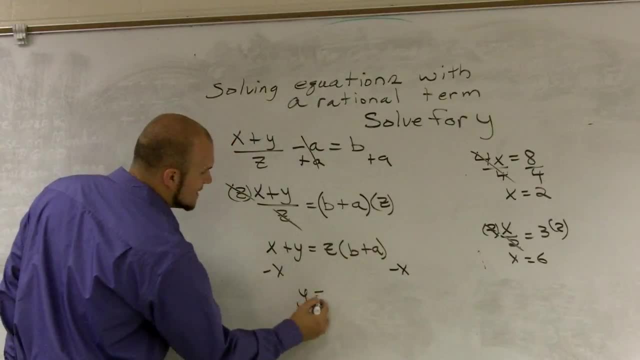 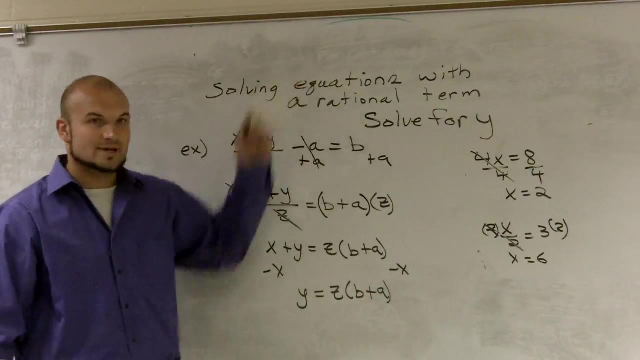 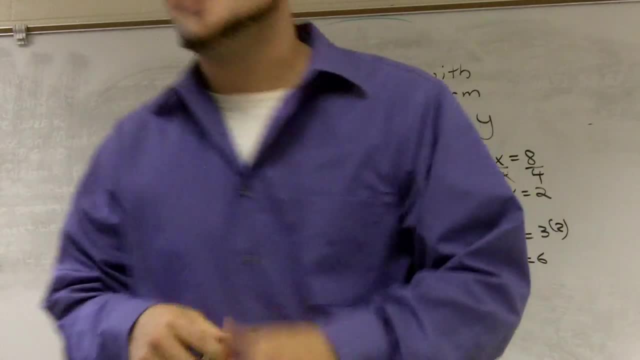 That's how you solve an equation with a rational term. I mess that up every single time.